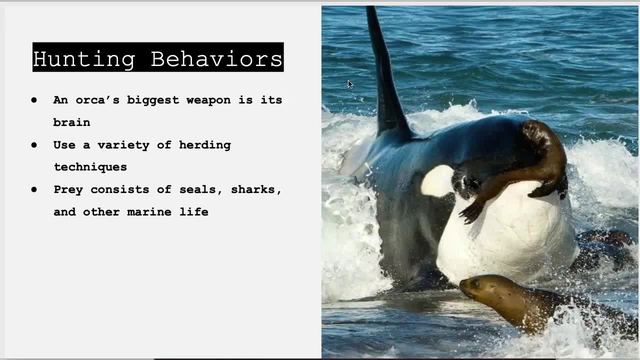 it's actually their brain which is the second largest among all marine mammals. This puts them at an advantage when it comes to hunting, which involves close communication to plan and execute coordinated attacks on their prey. Orcas use a variety of methods when catching their prey, including herding fish, drowning other whales and propelling themselves up onto beaches. 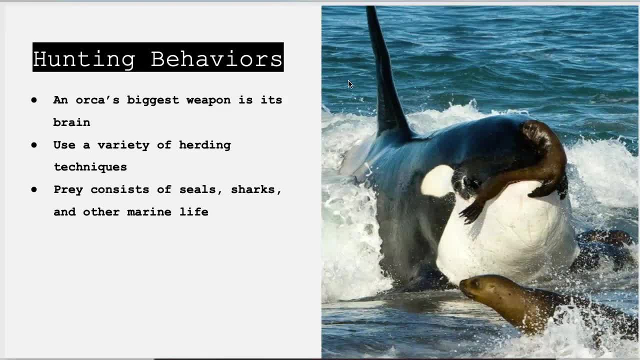 They use a karate chop technique to stun sharks, using their tail to slam into their head. Their diet consists of marine mammals: sharks, seals, octopus, fish, crustaceans, turtles and more. Since they are such strategic hunters, 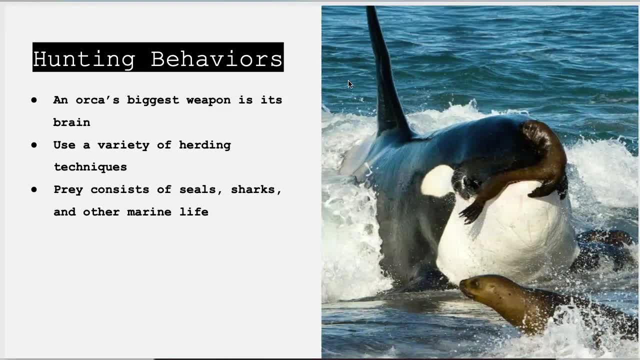 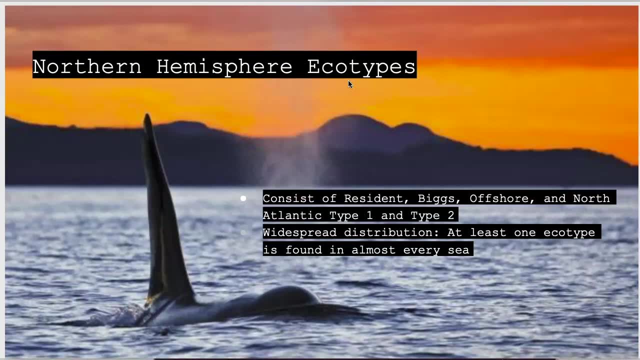 it takes the orca significantly longer to find prey than it does to catch The Northern Hemisphere. orcas are grouped into ecotypes: ecotypes meaning a distinct form or race of a plant or animal species occupying a particular habitat. The name of these ecotypes are resident, bigs, offshore and North Atlantic types 1 and 2.. 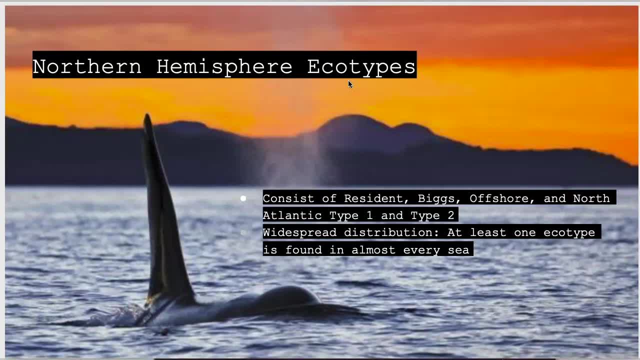 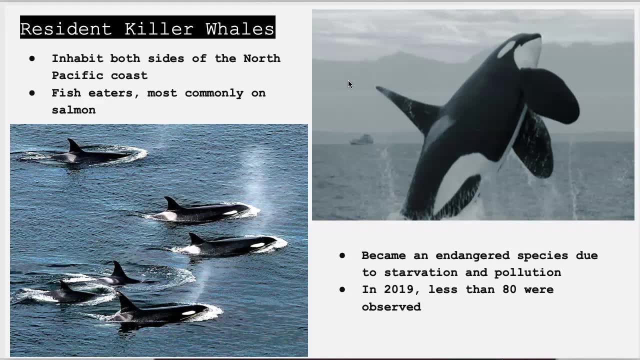 Each of these groups has specific habitats and diets. Resident orcas are known for training their prey and for the purpose of possessing the most of the animal's habitat, traits like belly rubbing or having a family-centered hierarchy. They live on both coasts of the North Pacific Ocean. Their diets consist mainly of salmon, but populations in 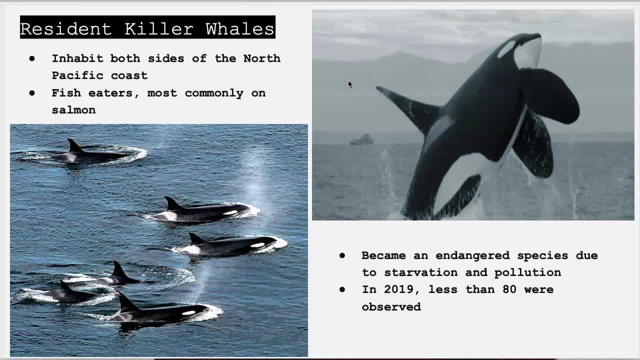 Alaska eat all types of fish. Residents stay with their family groups and travel in a community pod. One distinct feature of this ecotype is that their offspring live with their mother for their entire lives. Unfortunately, the species have become endangered due to diminishing salmon populations. 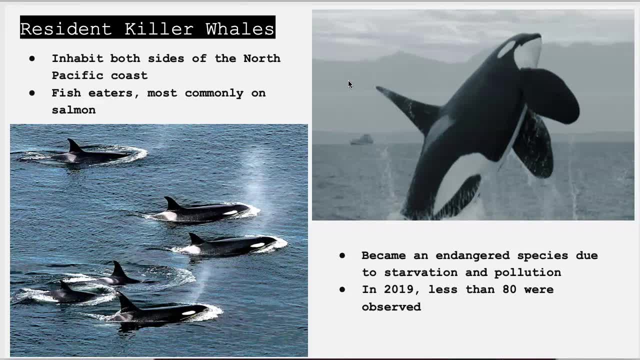 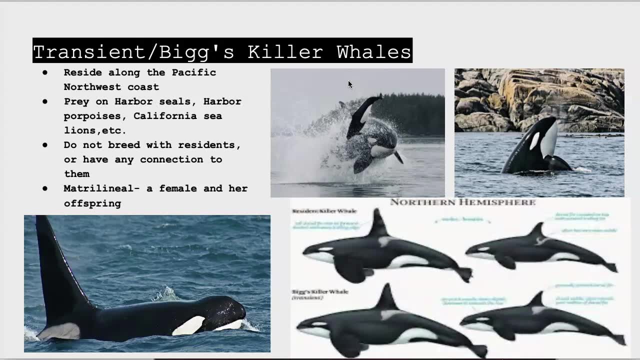 and pollution. In 2009,, a study showed there were less than 80 individuals left in the wild. Next are the transients, or bigs. They also reside in the North Pacific, but are found more northwest. They prey on harbor seals, harbor porpoises, California seal lions and other. 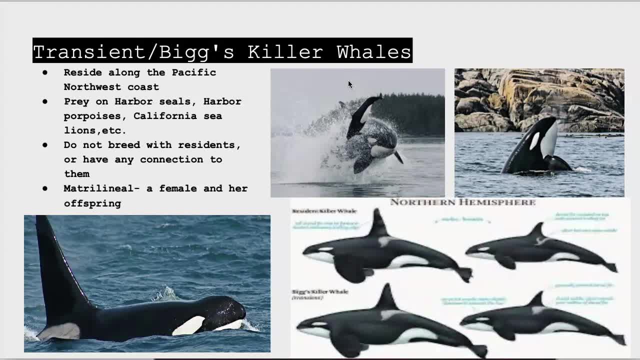 animals like calves of gray whales. It is said that they like to travel in small groups, which is odd for orcas. Like residents, they are known to have a hierarchy pod structure, Even though they are very similar in appearance to resident orcas. these two types of ecotypes do not breed. 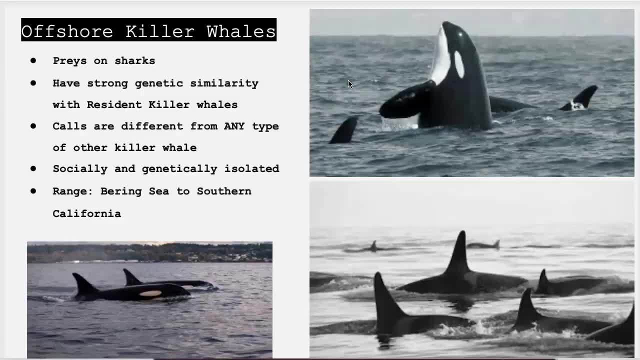 or communicate with each other. The next type of orca is the offshore form. It is found offshore from California to the Bering Sea, typically seen over the continental shelf. Physically, they are the smallest of the northern hemisphere orcas and are most closely related to the resident orcas- Their food. 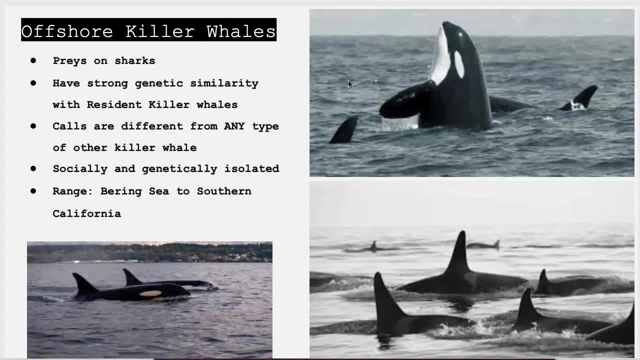 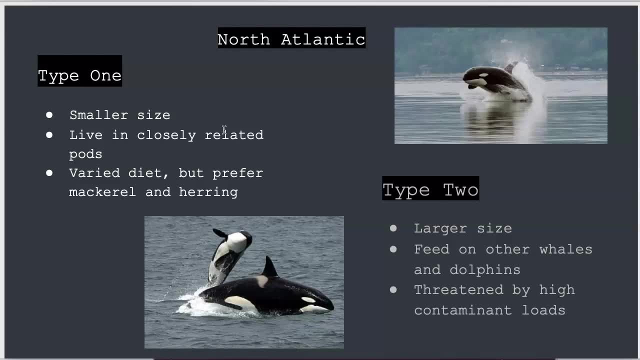 preference is unknown, but it's believed that sharks are a part of their diet, since their teeth tend to be worn down. Lastly are the Atlantic types 1 and 2. Type 1 is smaller and these whales eat whatever they can find, but they prefer mackerel and herring. 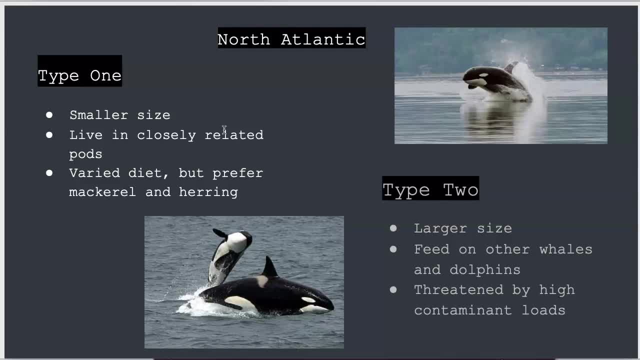 Some in Norway are known to eat seals. Type 2 is larger and these prefer to feed on other whales and dolphins. They have long, sharp teeth for digging and ripping into the flesh. A distinctive feature of this ecotype are the saddle patches behind the dorsal fin. Both of these groups are 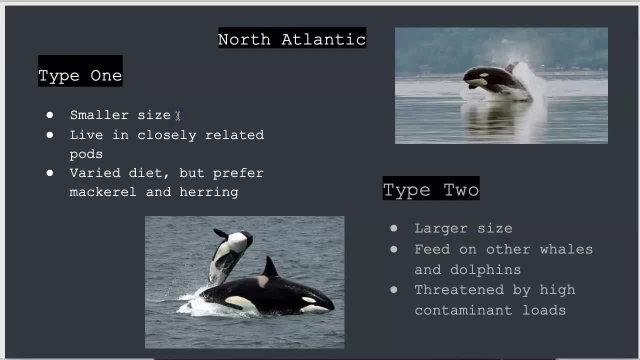 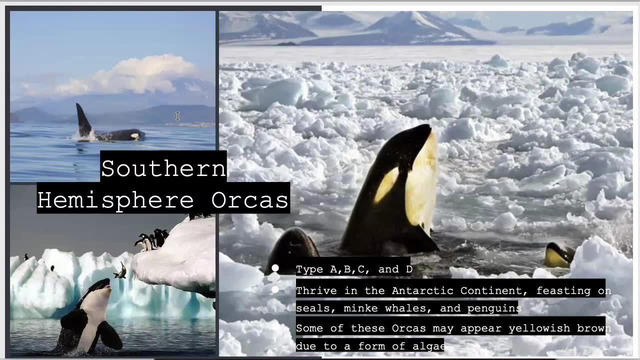 threatened by pollution and human activities. Southern hemisphere orca whales live in the Antarctic region. There are four types: A, B, C and D. Each exhibit slight variations in appearance. Their diets consist mainly of seals, mink whales and penguins. 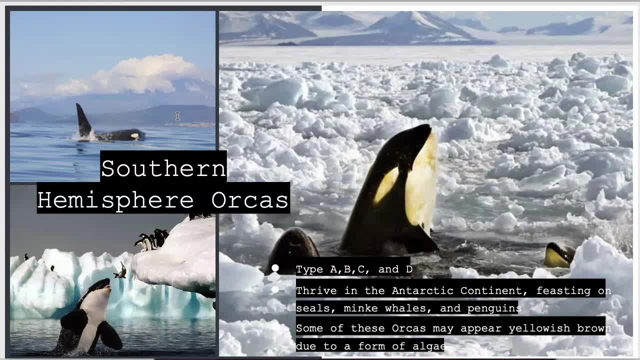 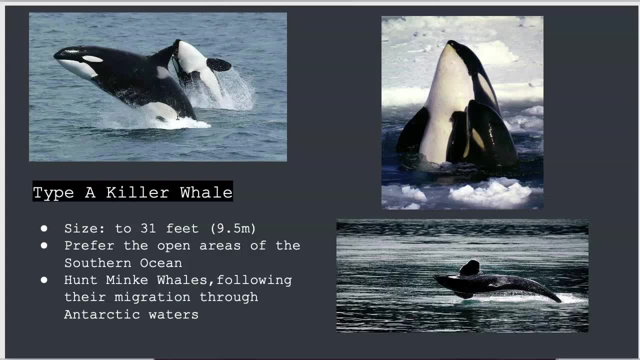 Due to algae called diatoms that grow profusely in polar waters. the skin of some of these ecotypes often display a yellowish tone. Type A orcas prefer the open ocean and southern waters, typically between latitudes 40 to 60 south. 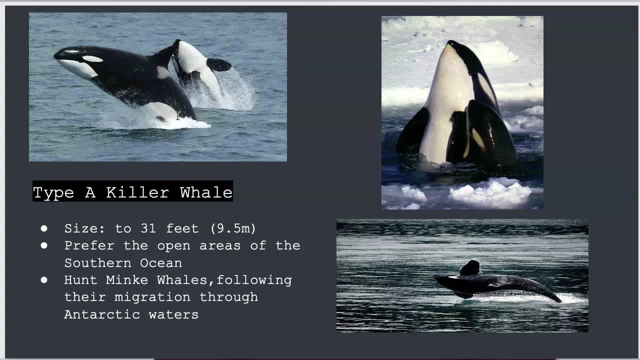 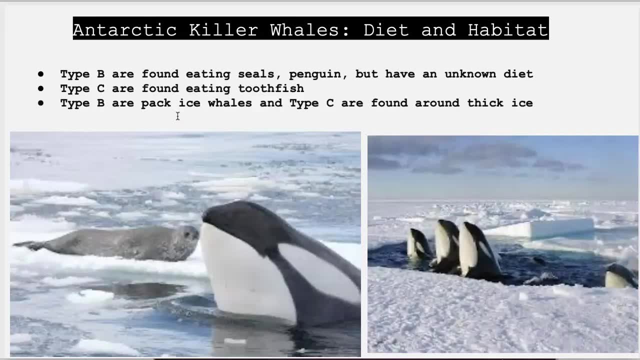 but they migrate to coastal Antarctic waters to hunt mink whales. They can grow to be humongous marine mammals up to 31 feet or 9.5 meters in length. Type B orcas are sighted on the Antarctic Peninsula and are considered iconic. Type B orcas are sighted on the Antarctic Peninsula and are 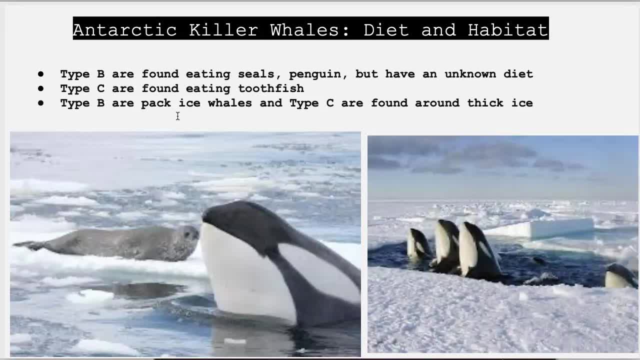 considered iconic. Type B orcas are sighted on the Antarctic Peninsula and are considered iconic. Type C orcas are sighted on the Antarctic Peninsula and are considered iconic. Type B orcas are sighted nada on snow and then died. inessionies inoculated with many large 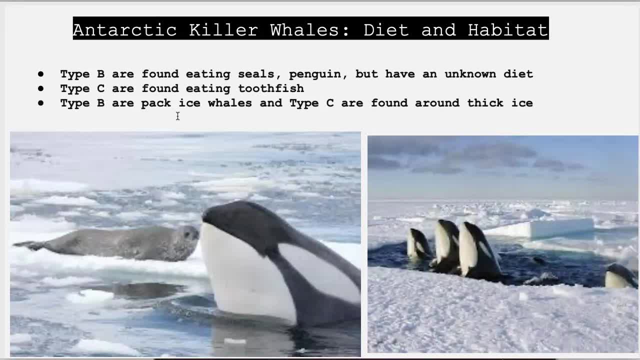 very large terrestrial facilities. They generate very trapped clothes, healthy skin, as close to their core body as possible as markers do. Type C orcas are sighted on the Antarctic and whiteück oak akan five, 그때ki two oaks and then called the